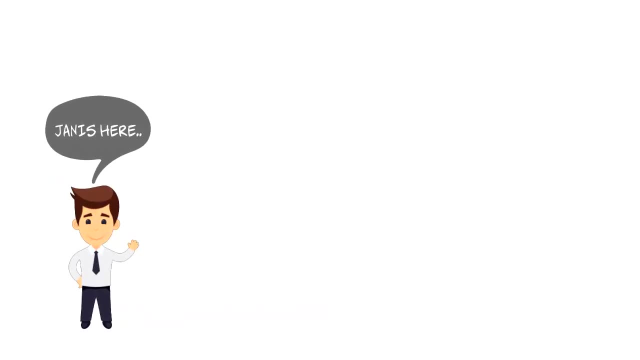 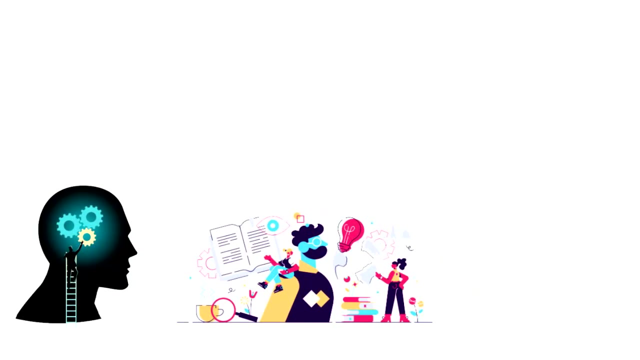 Hi everyone. it's Yanis here, and in this video we will explore what is cognition. Your highest brain functions operate subconsciously, but they are important and you need to make sure that you nurture them. If this is your first time on this channel, then make sure you subscribe and 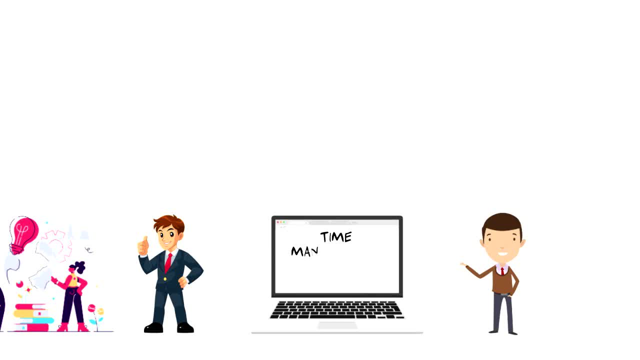 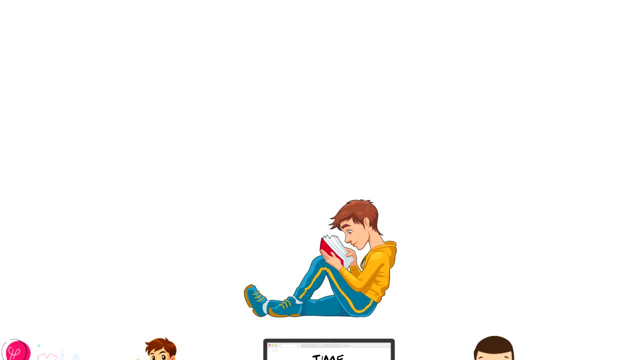 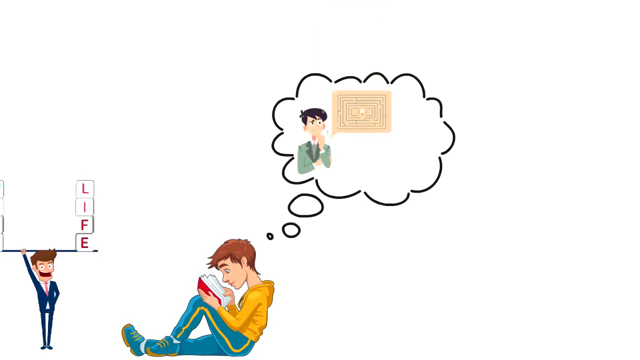 hit the bell icon to get updates on my latest videos about time management and productivity. Cognition refers to the mental process of acquiring knowledge and understanding through thought, experiences and senses. These cognitive processes include attention, thinking, the formation of knowledge, remembering, judging and problem-solving. These are higher-level 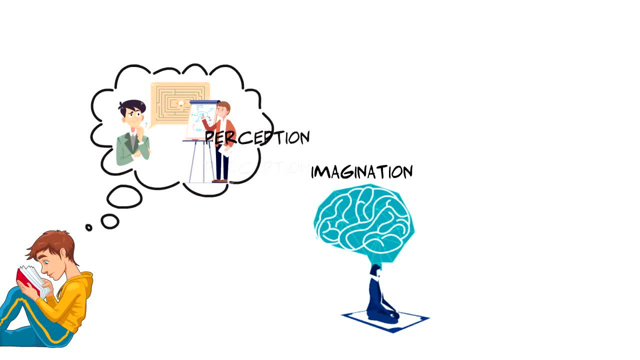 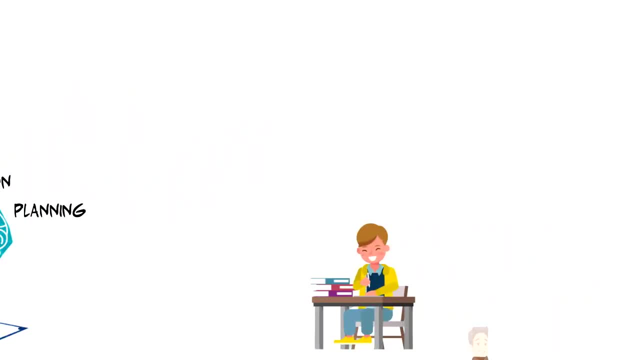 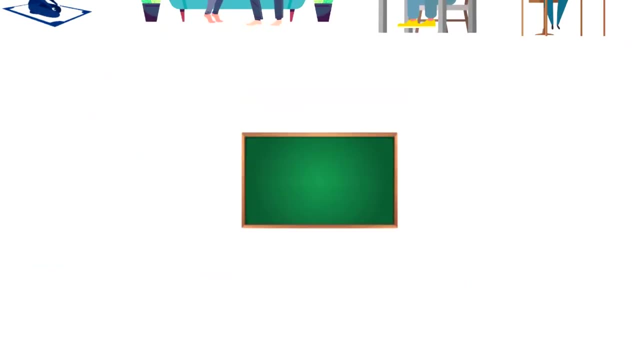 functions of the brain and encompass language, imagination, perception and planning. Cognitive processes affect every aspect of life, from studies to work to relationships. Some specific uses of these cognitive processes include the following: First learning: Learning requires you to take in new information and combine with existing. 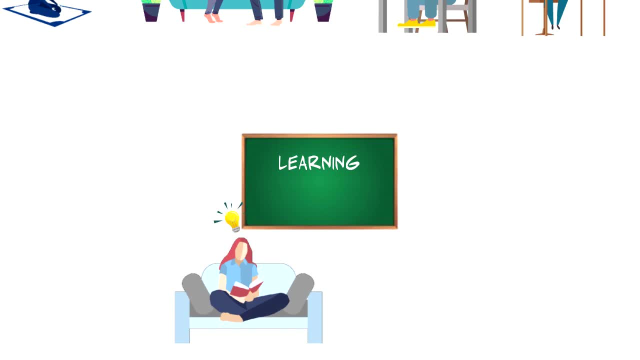 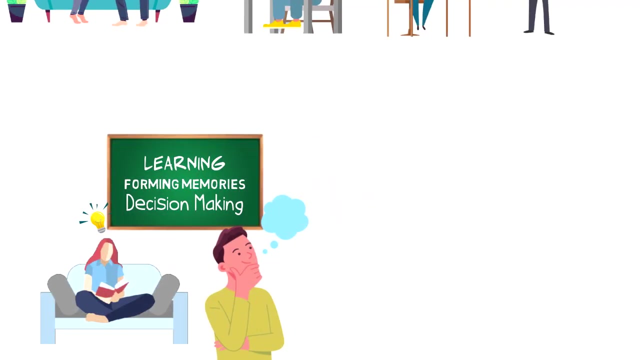 information to form new concepts and understanding. Second, forming memories: How we remember, what we remember and what we forget reveal a great deal about how the cognitive processes operate. Third, decision-making. Whenever you are making a decision, you have to evaluate. 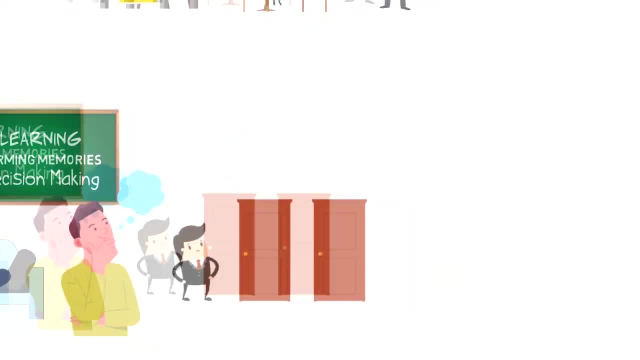 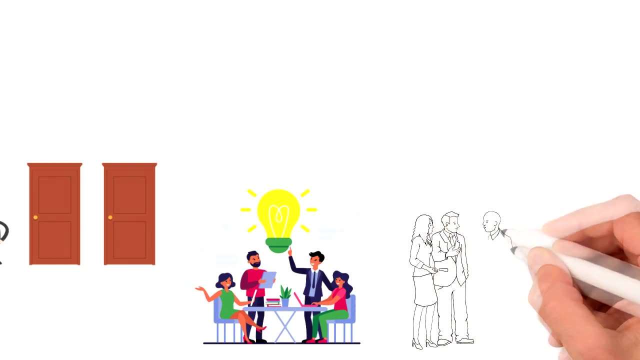 the information that you have and judge it based on your knowledge. Our cognitive abilities are extremely important as they impact how we perceive the world, form impressions and interact with our environment. That's why you have to nurture your cognitive abilities. Here are some tips. 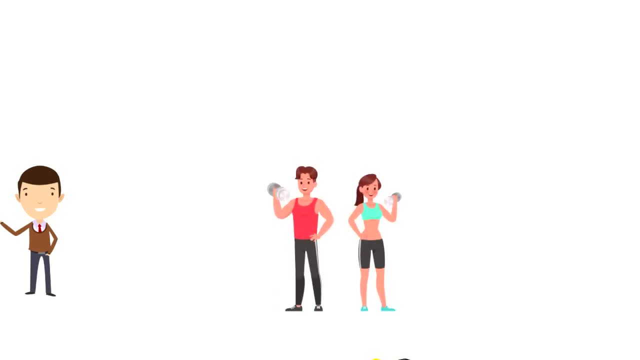 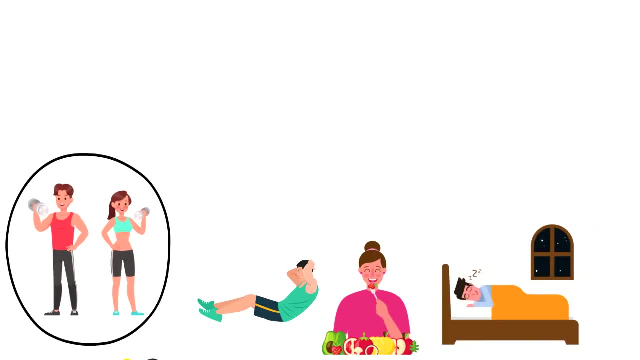 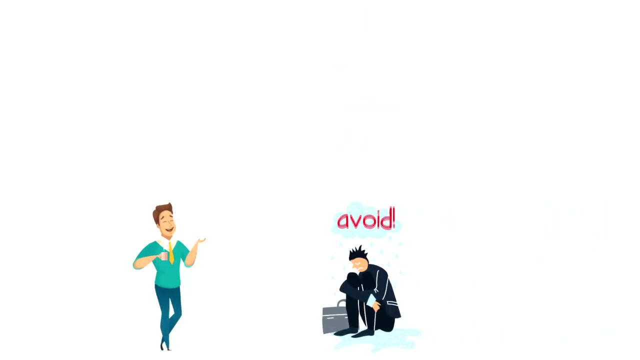 on how to do that. First, stay healthy. These are the basic human needs: Exercising, eating healthy foods for most of the time and having a good sleep. Second, reduce stress. Stress has a negative impact on your brain function and therefore it is important to avoid it. Plan your 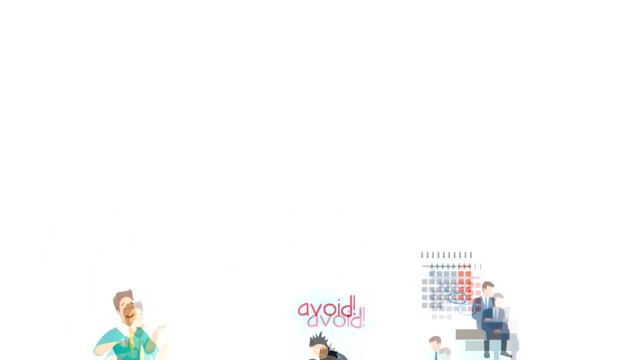 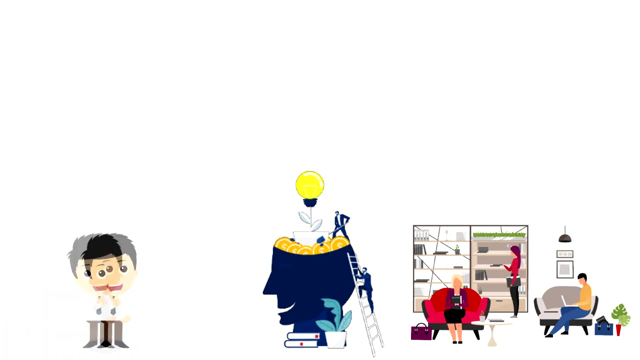 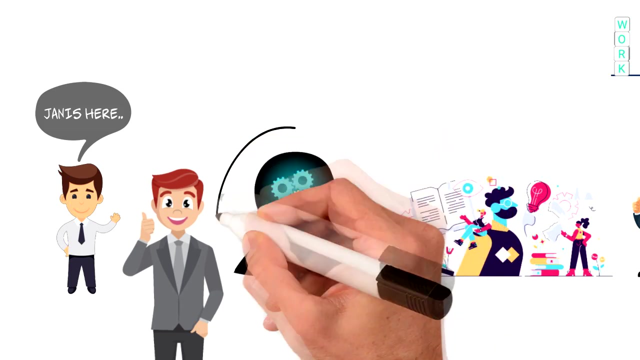 time accordingly, so you don't have to stress about uncompleted things. Third, keep learning To exercise and develop your cognitive functions. you have to consume new information, so make sure that you keep learning new things. I hope that you enjoyed this video and I was able to give you a